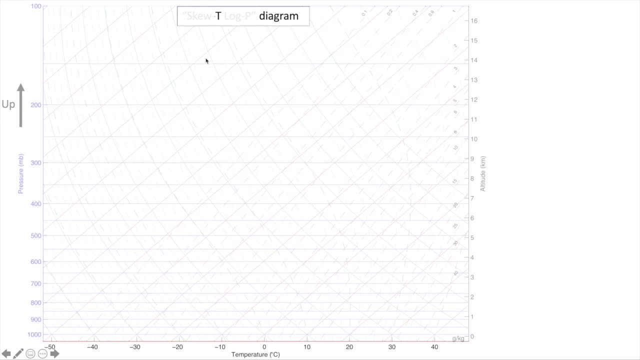 So the first two are in the name of the diagram. The T in skew-T refers to temperature, which is our horizontal axis and spans the typical range of temperatures observed in the atmosphere from about negative 50 to 50 degrees Celsius, And the P in skew-T, log-P, refers to pressure, which is our vertical axis, where up can literally be interpreted as being up in the atmosphere. 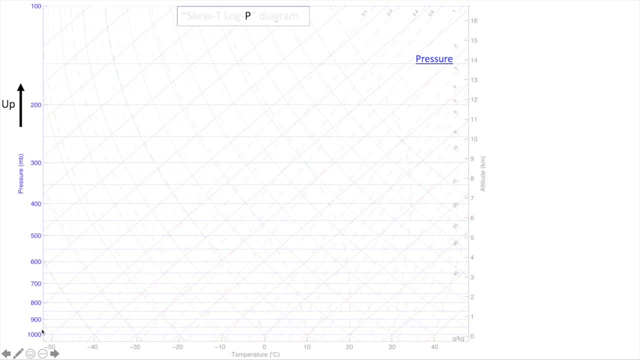 This pressure axis ranges from typical sea level pressures of around 1000 millibars to pressures typical of the upper troposphere or lower stratosphere. The log in log-P refers to the fact that the pressure axis is scaled logarithmically, which can be seen by these 100 millibar intervals increasing in spacing as you go up the vertical axis which we are thinking of as up in the atmosphere here. 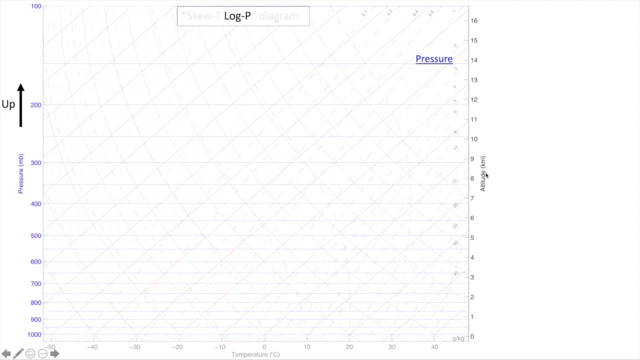 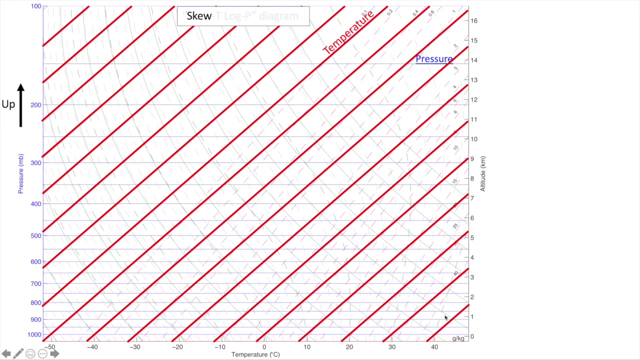 We can see that these logarithmic decreases of pressure correspond to linear increases in altitude, in terms of distance, which we can see on the right vertical axis. The skew in skew-T refers to the pressure of the atmosphere. This is a reference to the fact that the lines of constant temperature, or isotherms, are skewed 45 degrees clockwise, which is mostly done out of convenience so that we can plot a wider range of temperatures in a more compact space. 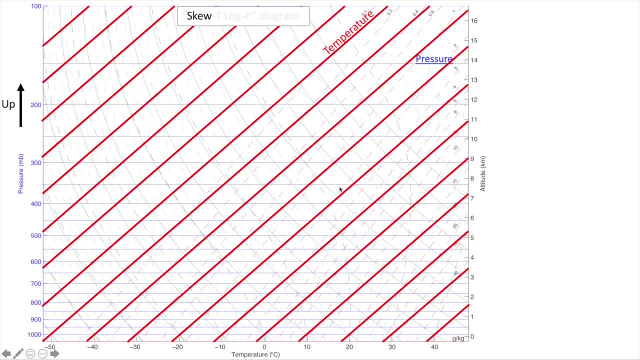 But this skewing makes these charts a little counterintuitive for those who have not worked with them before. So, for example, if we imagine that we measure temperature going up in the atmosphere and it looked like a vertical line on this diagram, our first intuition might be that temperature is constant with height. 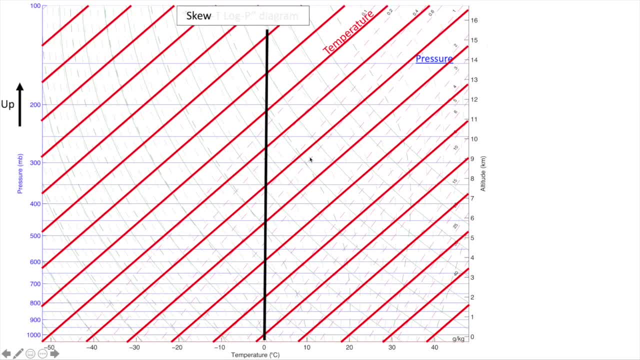 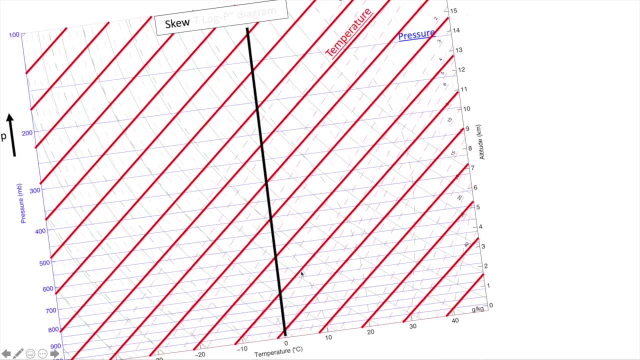 But the P in skew-T log-P refers to the temperature of the atmosphere. this is not the case. Instead, we can see that we are continuously crossing lines of constant temperature, and thus temperature is decreasing with height. It may be easier to see this if we momentarily unskew the temperature axis. 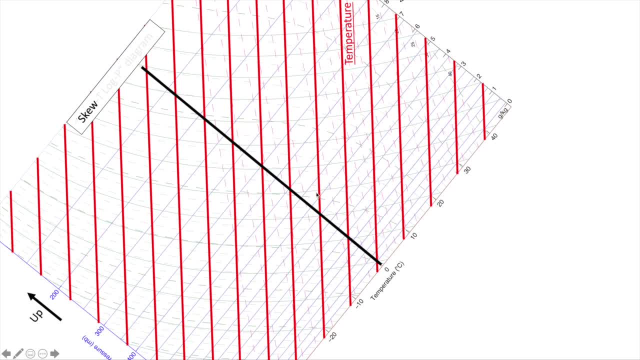 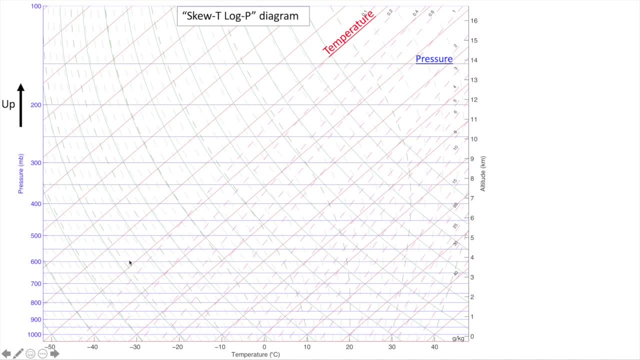 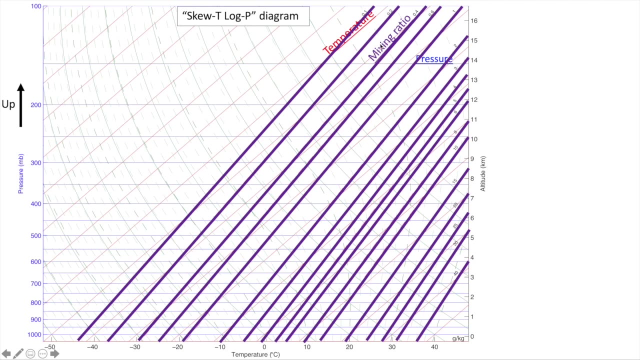 showing a negative slope in our hypothetical measured temperature. So this is a temperature pressure space, and thus we have one set of lines representing temperature and one set representing pressure. but we have three more sets of lines to explain The first of the remaining set of lines that we 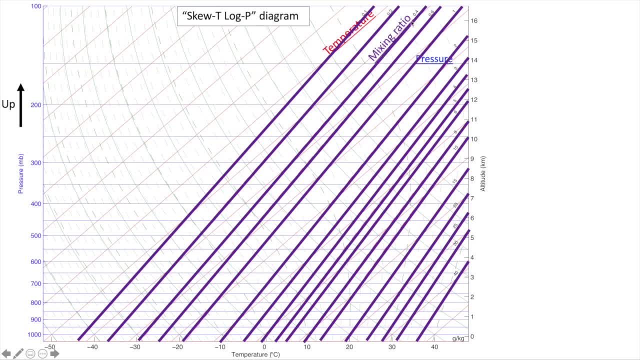 will explain. is water vapor mixing ratio or the ratio of the mass of water vapor in the air to the mass of everything else in the air, which includes nitrogen, oxygen, argon, increasingly CO2, etc. And this is in grams per kilogram. When 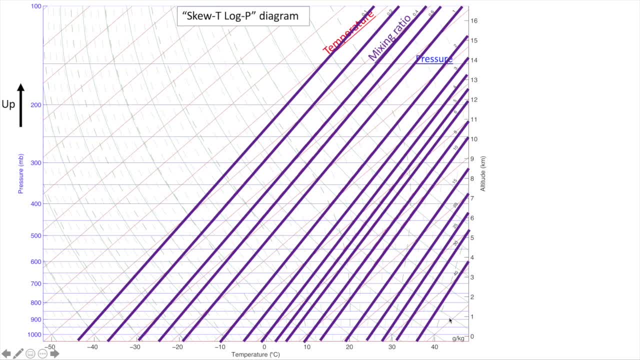 mixing ratios are plotted in this temperature pressure space. they're telling us how much water vapor can be contained within a parcel of air of a given temperature And pressure. This is known as the saturation mixing ratio. So a parcel of air with a pressure of 700 millibars and a temperature of 15 Celsius would 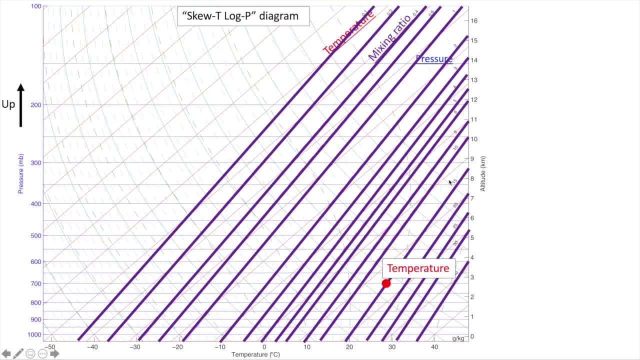 hypothetically be able to support as much as 15 grams of water vapor for every kilogram of dry air. Another way of saying this is that at 15 grams of water vapor per kilogram of dry air, this air parcel would become saturated and any 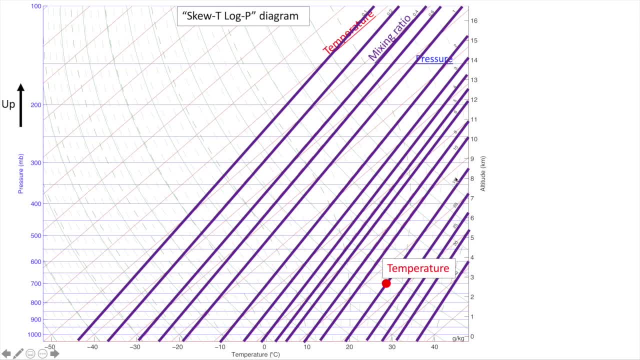 additional water vapor added to the parcel would condense in form clouds. We can see that at the coldest temperatures on the diagram, the atmosphere will have a capacity to contain only a very, very small amount of water vapor, and at the warmest temperatures in the diagram, the 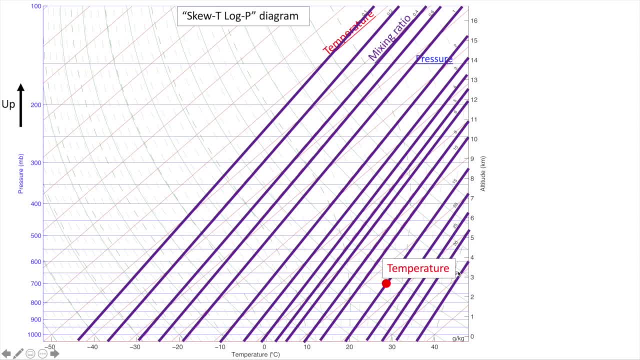 atmosphere can accommodate around 40 grams of water vapor per kilogram of dry air, or close to four percent of the atmosphere by mass. Now if, in addition to the temperature, we also measure the dewpoint temperature of this hypothetical parcel of air, we can plot that in this temperature pressure space. 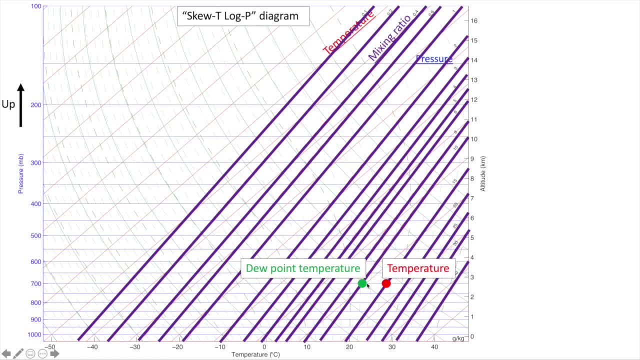 space as well. The dewpoint temperature is telling us the amount of water vapor actually in that parcel of air, in this case, 10 grams per kilogram. This means that this parcel is subsaturated, since it contains less water vapor than it would possibly be able to accommodate. It contains 10 grams per 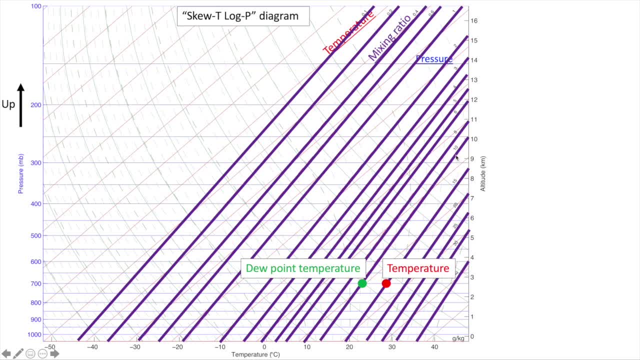 kilogram, but it can potentially accommodate 15 grams per kilogram. This ratio, by the way of 10 grams per kilogram divided by 15 grams per kilogram, is the definition of relative humidity, which is thus around 67 percent in this case. Now, the other two sets of lines are both: 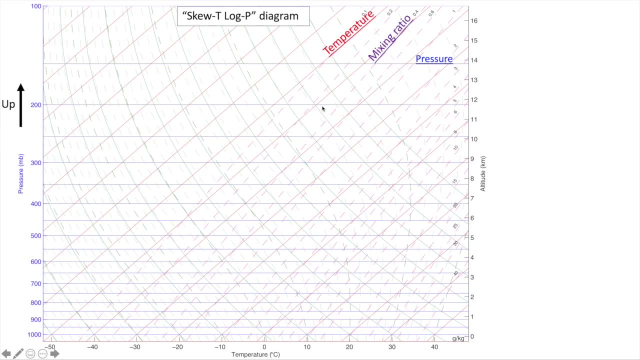